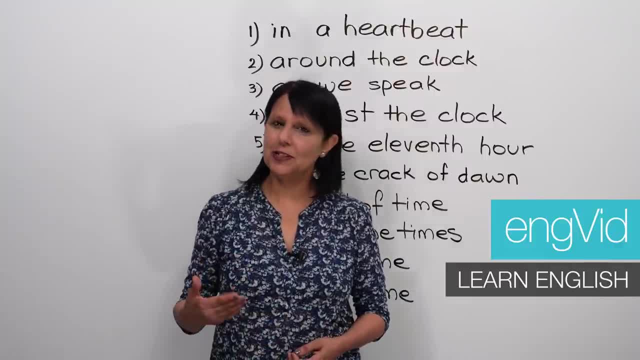 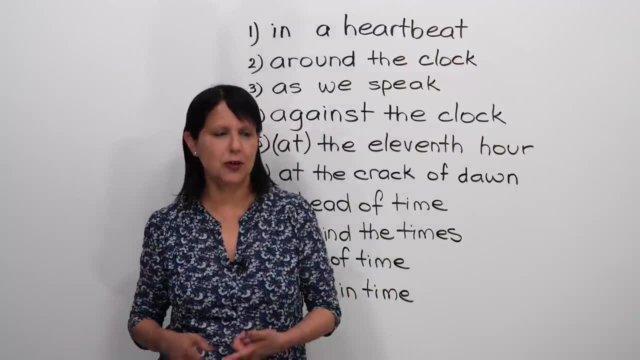 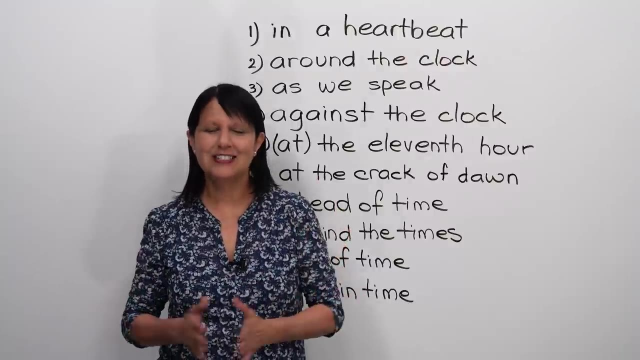 Hi, I'm Rebecca from engVid. In this lesson you will learn ten idioms of time, So these expressions are used in all kinds of situations, whether they're general, whether they're social situations or business context. You might hear them anywhere, So it is very useful. 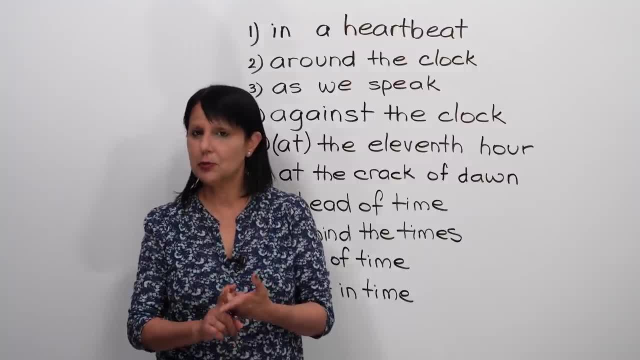 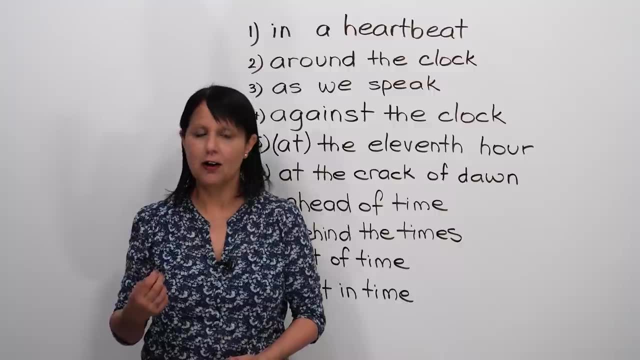 to be able to understand them first of all. That's the most important thing you want to be able to do when you learn idioms, and then, when you're really sure of the meaning and how to use them, you can also start to use them yourself. Okay, So let's look at 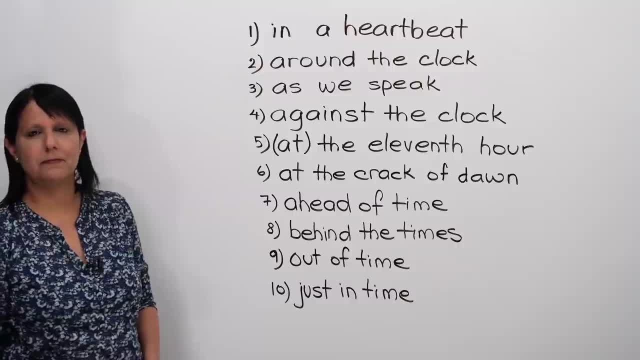 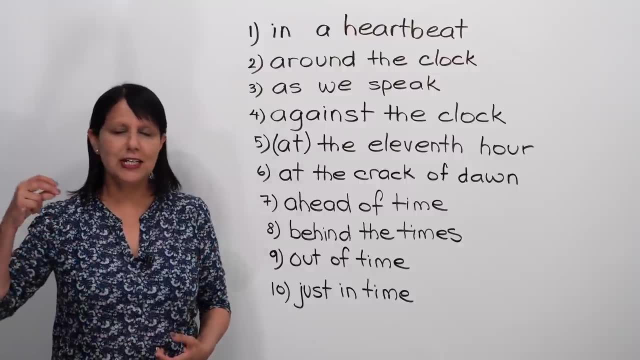 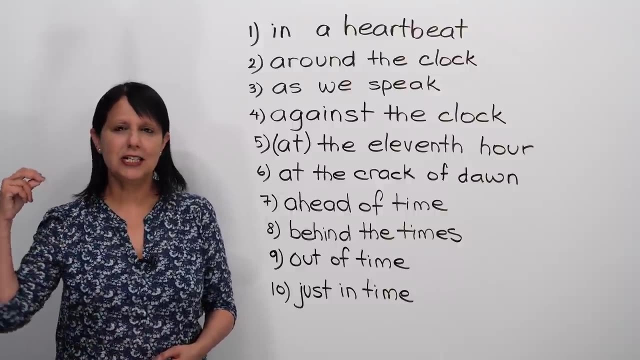 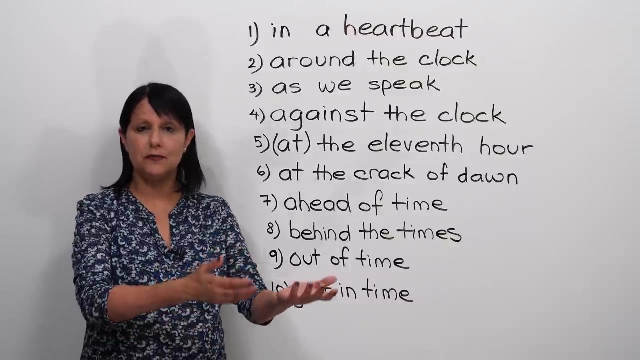 what they are. So the first one: in a heartbeat. Let me give you an example: Life can change in a heartbeat. So what do you think that means? It means life can change in a heartbeat, Immediately, Instantly, For example, right now. you decided to watch this video instead. 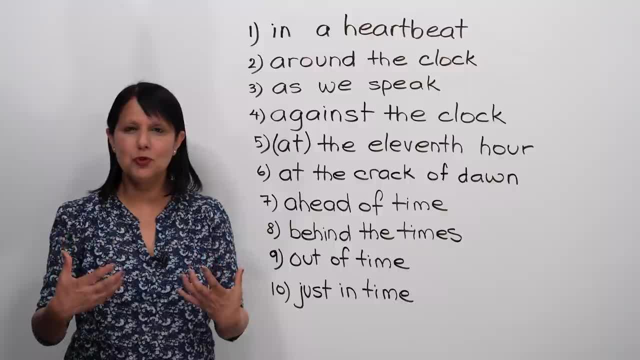 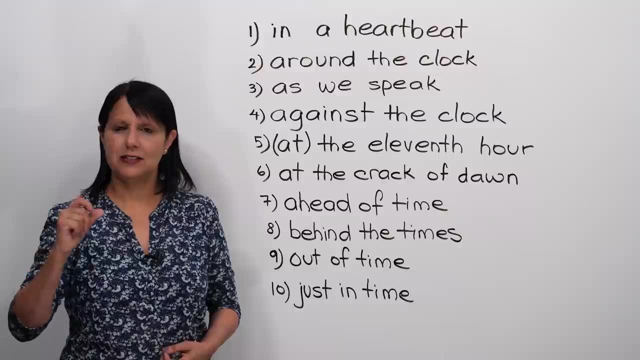 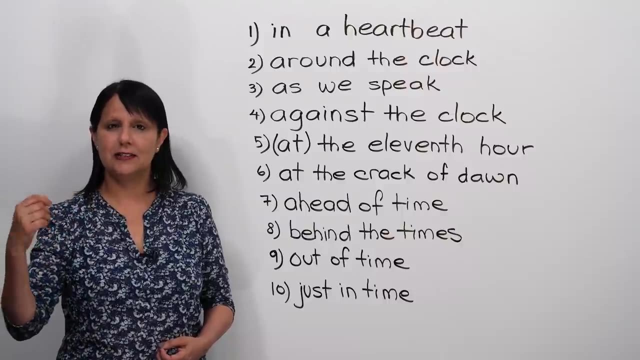 of doing something else. You decided to improve your English in a heartbeat. Okay, You can make that decision in a heartbeat. Just like a heart beats fast, right, Beats very quickly, Not necessarily fast, but quickly. In the same way, this expression means quickly, Instantly. 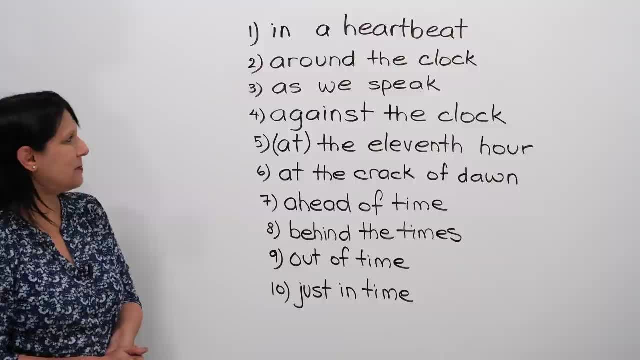 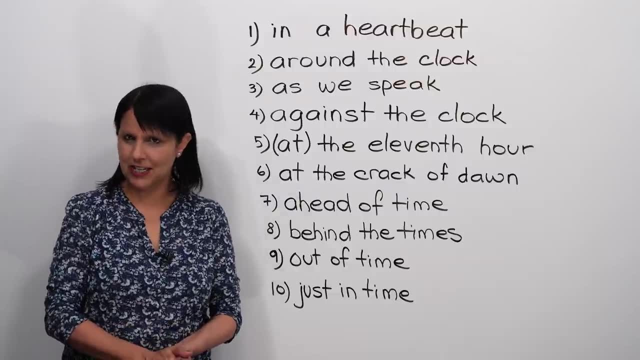 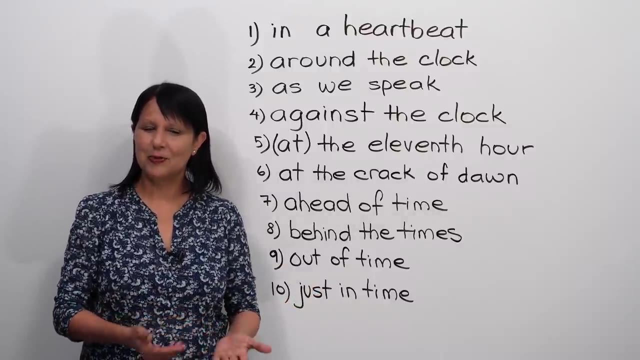 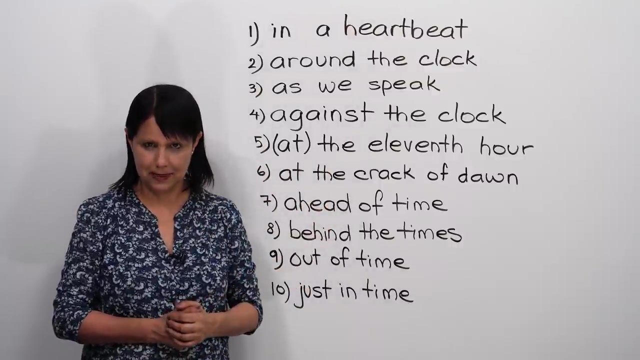 All right, Okay. Next Let's look at the next one, Number two: Around the clock. I'll give you a sentence. See if you understand. They deliver pizza around the clock. Okay, What do you think that means? Around the clock? So it means 24 hours a day, Okay, They deliver pizza at. 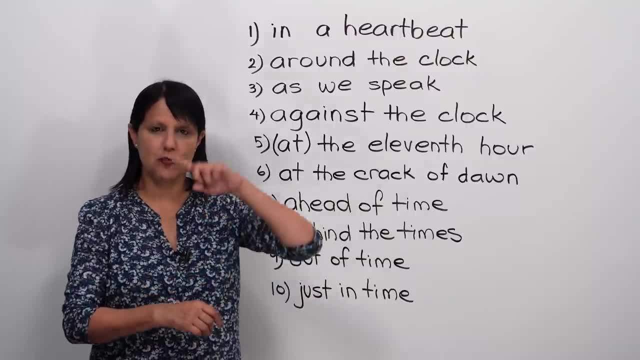 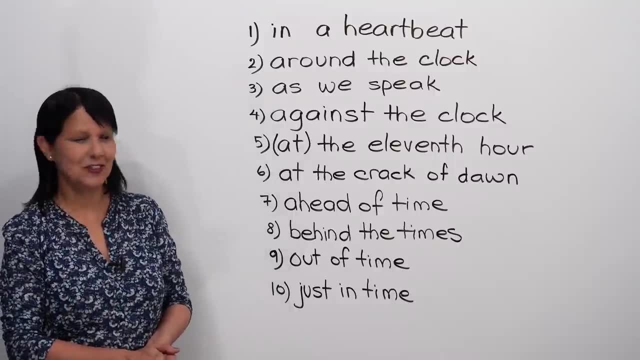 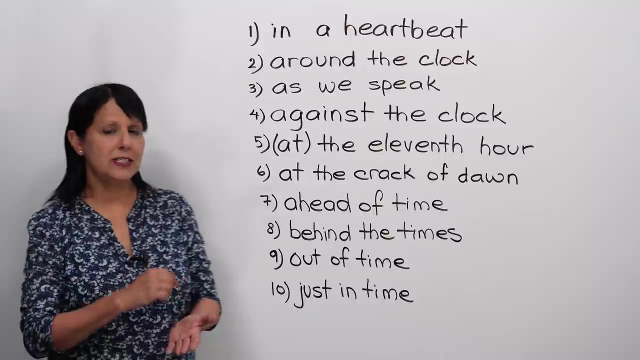 any time of the day or night, Around the clock. All right, That's the meaning of around the clock 24 hours a day. Good, As we speak. Let me give you an example. They are signing the deal as we speak. They are. 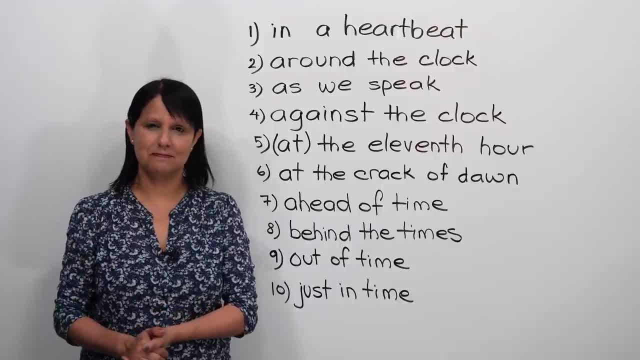 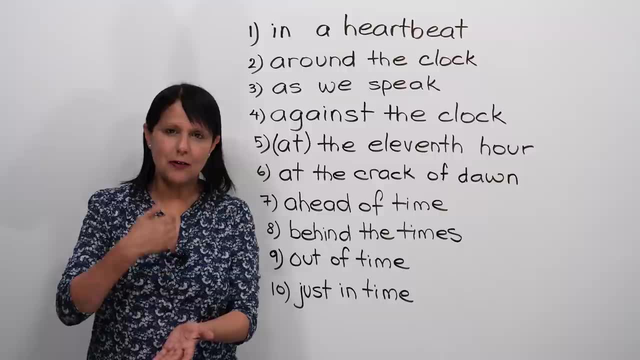 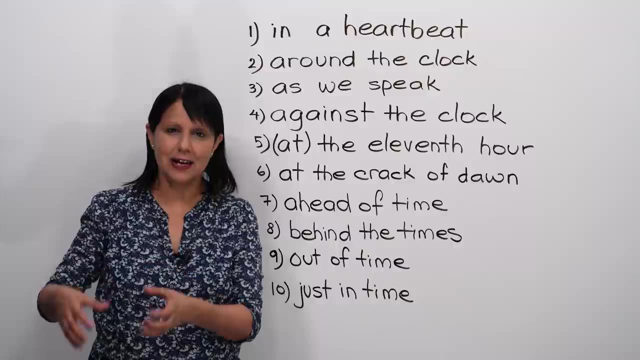 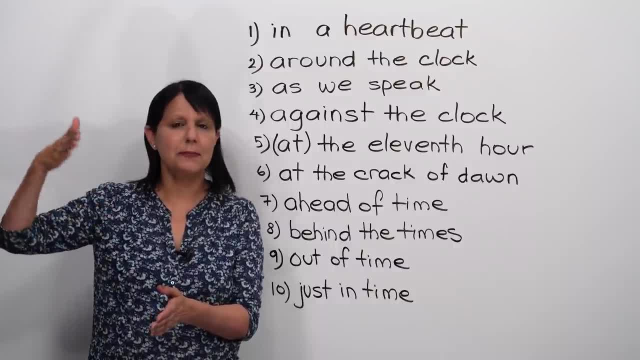 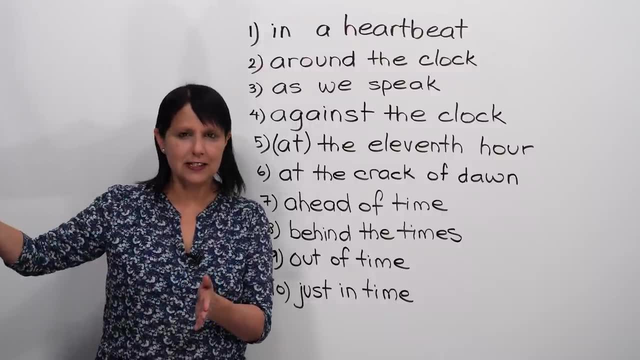 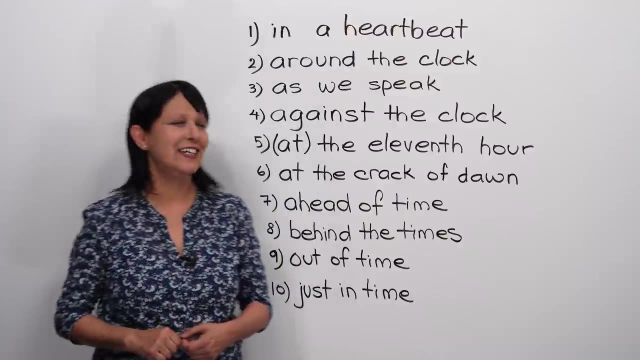 At this moment. Usually it's talking about something that's happening somewhere else while you are in one place. Okay, So, for example, they are signing the deal as we speak. That means as we are speaking. they are doing that right now. Okay, Let's look at number. 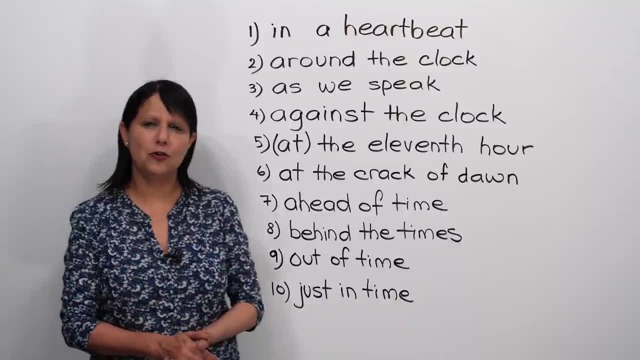 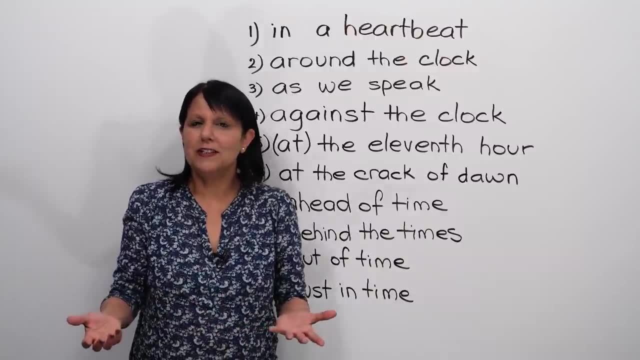 four: Against the clock, Against the clock, Against the clock. Okay, We are working against the clock to finish this presentation. All right, What do you think that means? And look at the way that I'm speaking. There's a little bit of 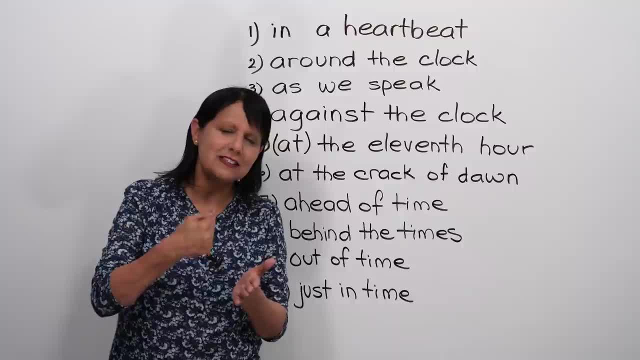 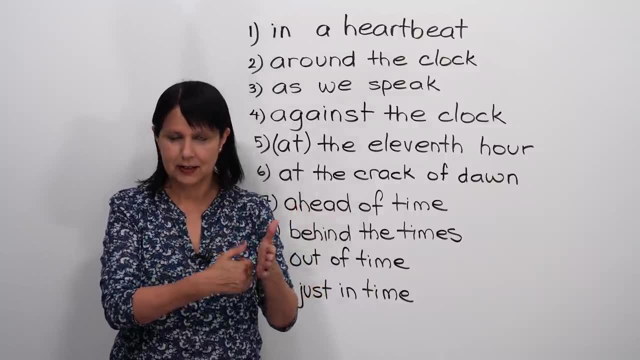 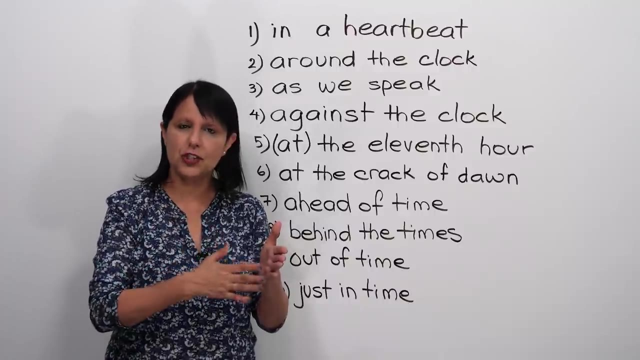 anxiety here, Right? So when you're working against the clock, you have a deadline and you're trying to finish something before that deadline, Before that time limit, Okay, So you're working against the clock, You're working really hard to finish something because you 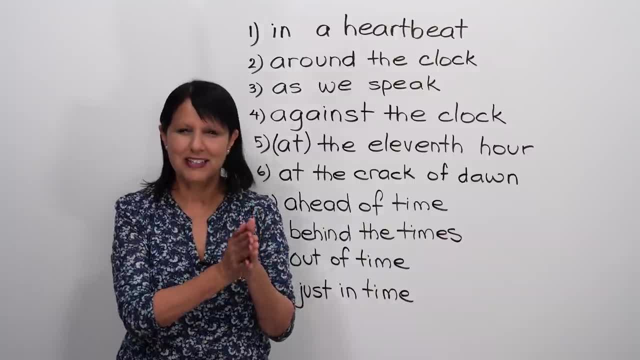 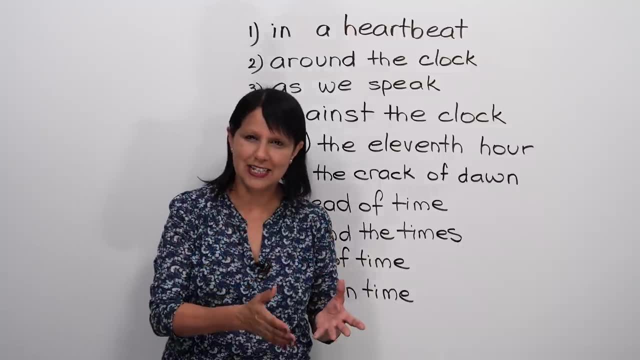 have a deadline and you have to finish by that time. All right, Let's say you have to get in an application by a certain time, or you have to finish a presentation by a certain time, because you're meeting your client in the morning, So you're working really hard. 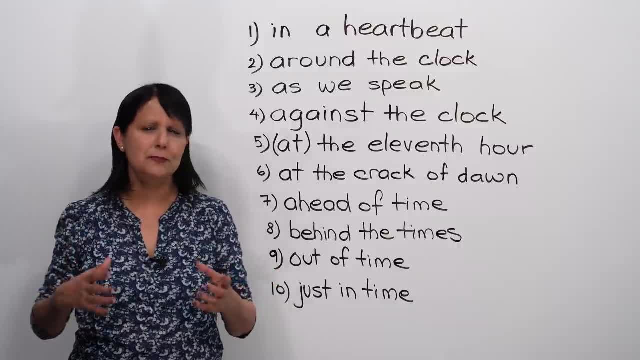 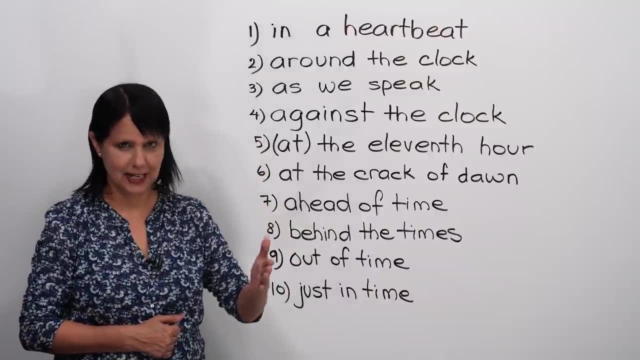 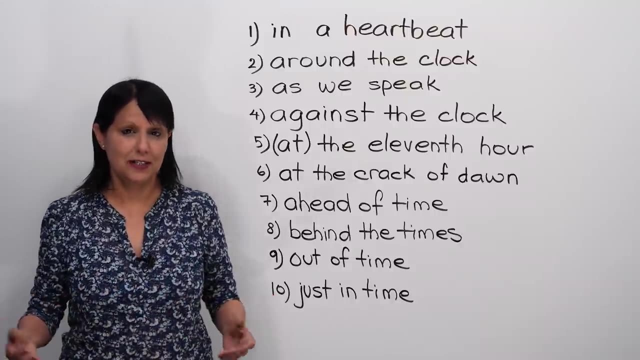 and you're working against the clock. You don't have enough time, You wish you had more time, but you're working against the clock. It means you're working to a deadline, All right, And at the eleventh hour or the eleventh hour. So let's say, Let's take this example forward. 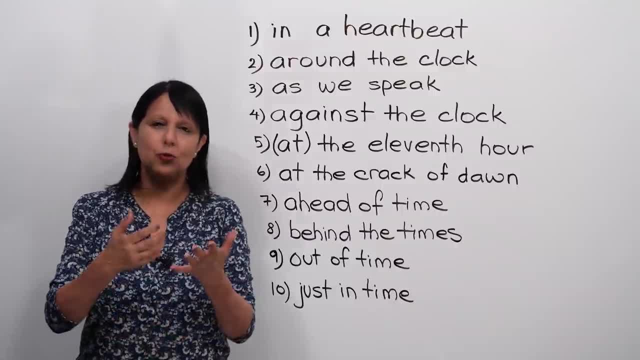 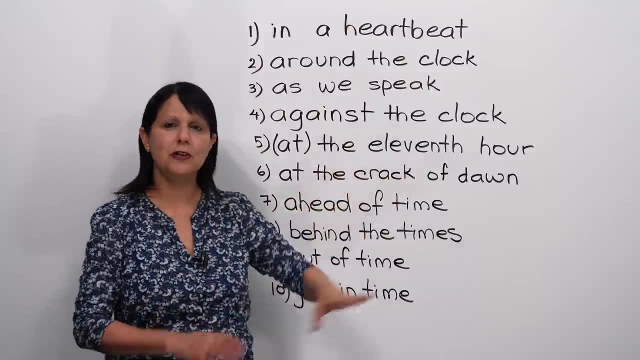 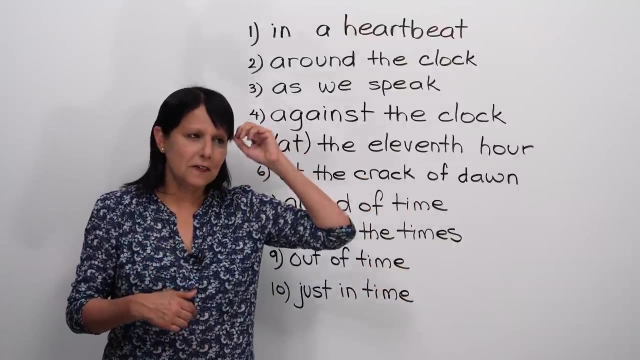 Let's say you were working against the clock all night long in order to finish your application or your presentation and then finally, at the eleventh hour, you finished everything, Okay. So what does that mean? At the eleventh hour means like just before the deadline, Okay. 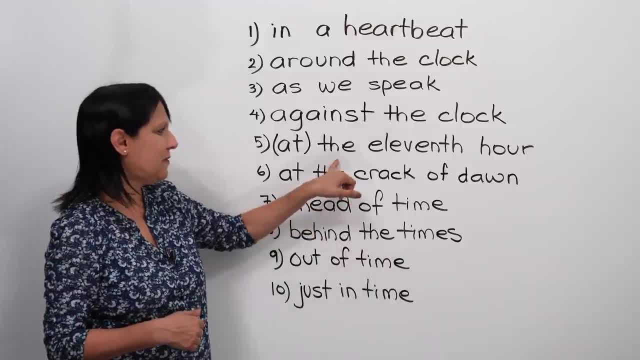 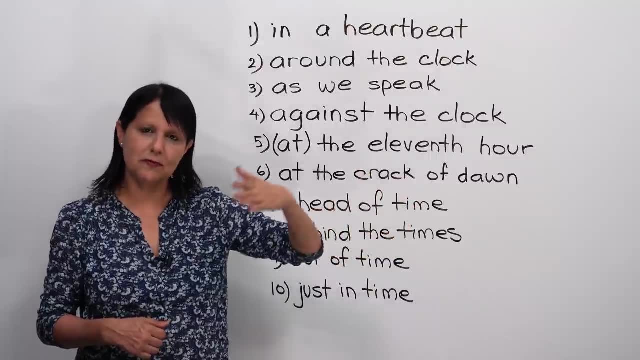 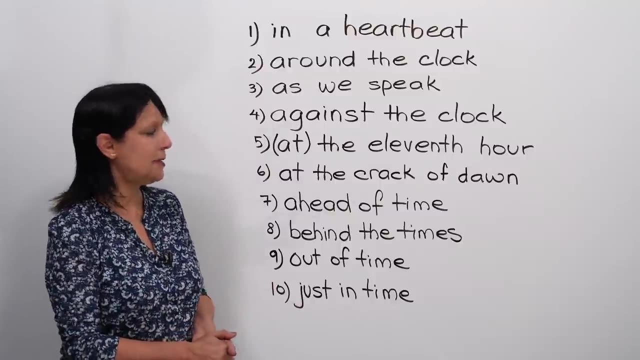 At the last minute. That's the meaning of the eleventh hour Okay, At the last minute, or just before the deadline, Just before the time limit. I finished it at the eleventh hour, Okay. Or you could say, for example, some students wait to study at the eleventh. 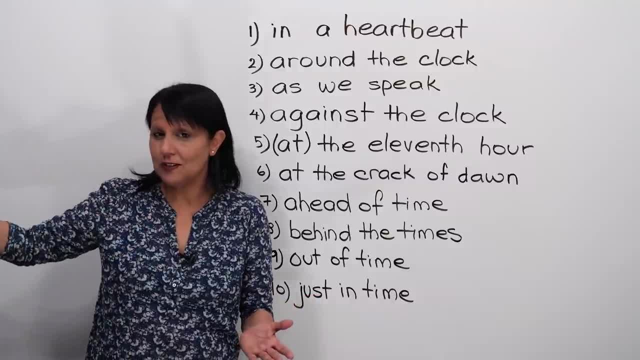 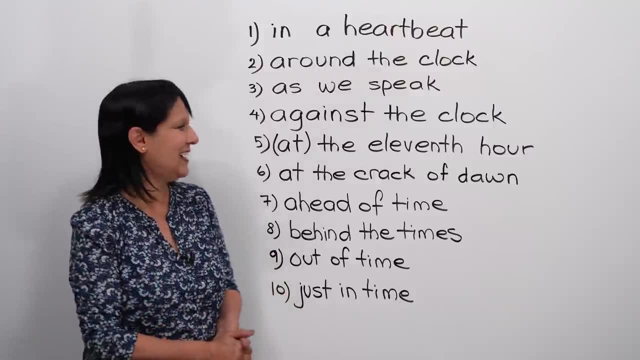 hour before an exam. They don't study all through the year. They wait till the eleventh hour to study really hard and crazy. Okay, So you're working against the clock, You're crazy, Not recommended, Okay, But it means they wait like till the very end. 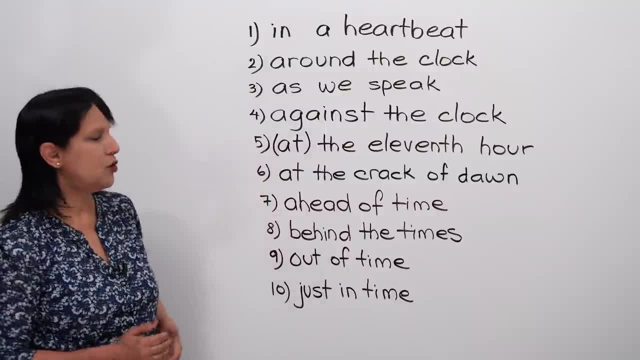 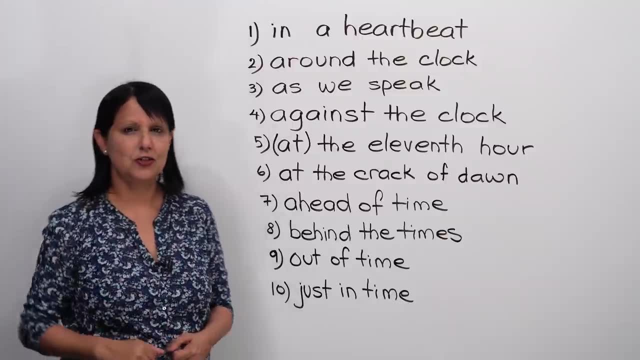 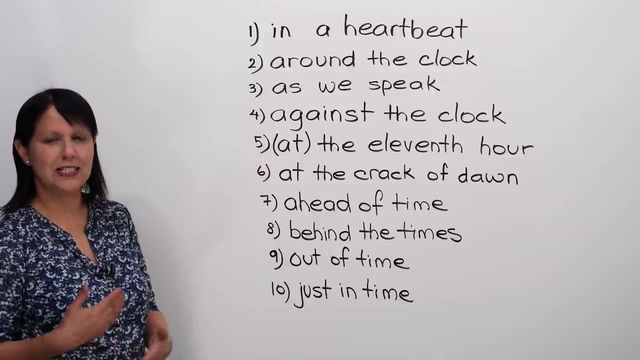 So let's review these first five, Okay? So if I want to say that something's happening right now, I'm talking to you and something's happening. So which one is that? Number three, Right As we speak, It's happening as we speak And suppose you say Things can change. 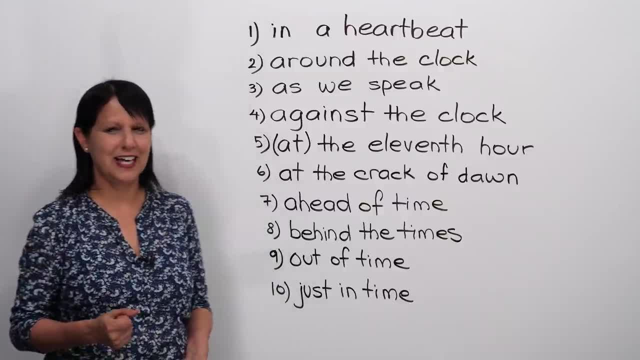 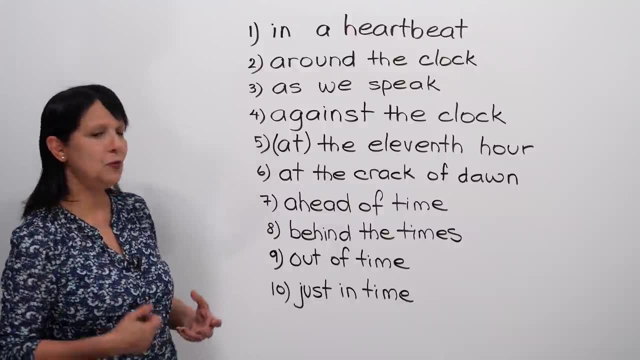 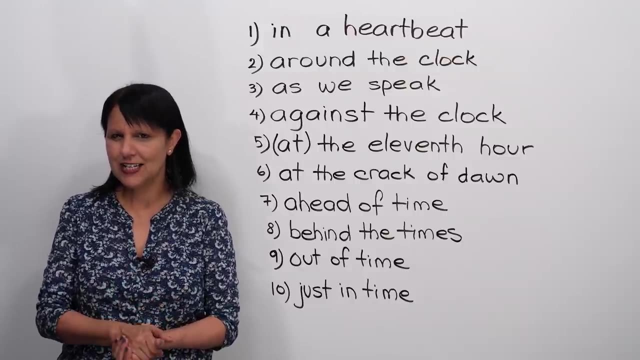 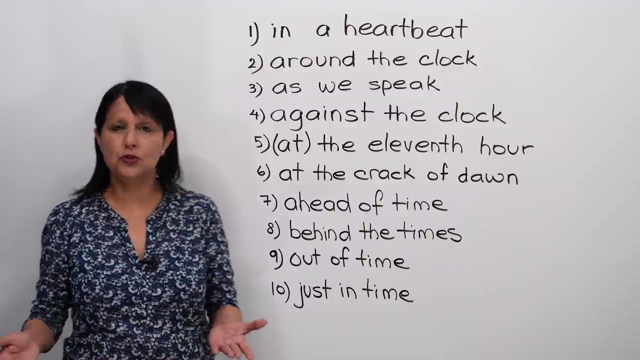 just like that, Which one is that Things can change in a heartbeat. Good, And if you want to say that you managed to finish something at the last minute, you could say: I finished it at the eleventh hour. Okay, And suppose you want to order pizza, So you're going. 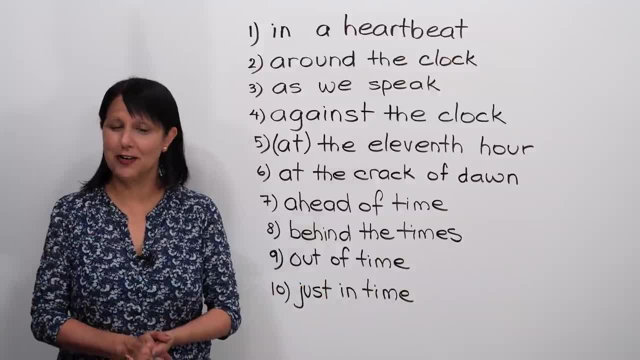 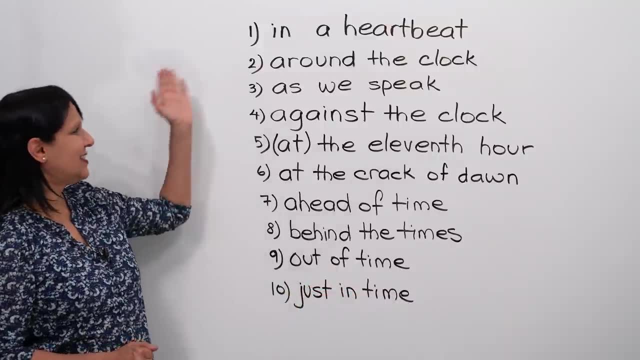 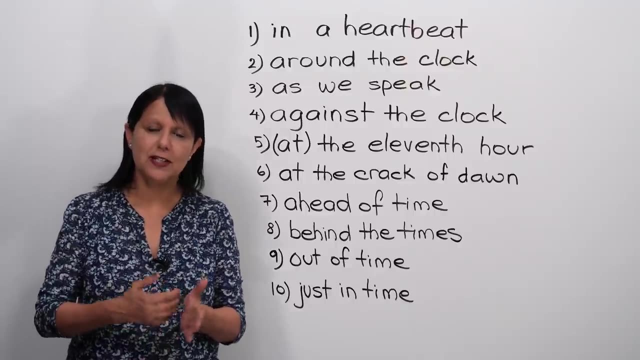 to 3 o'clock in the morning. so you're looking for a restaurant that delivers at any time, that delivers around the clock, right, Good? And let's say you're under pressure to finish something before a deadline, so you are working. 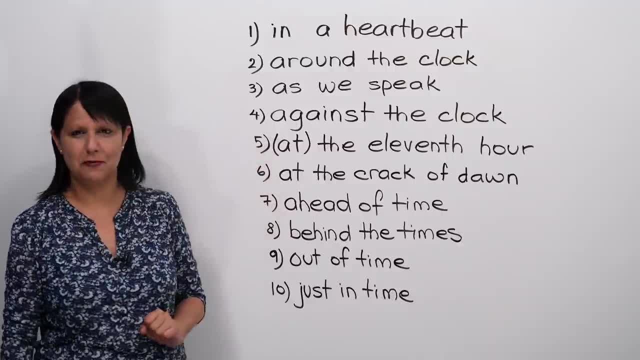 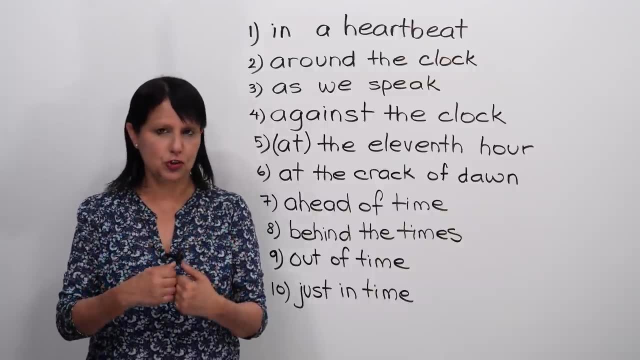 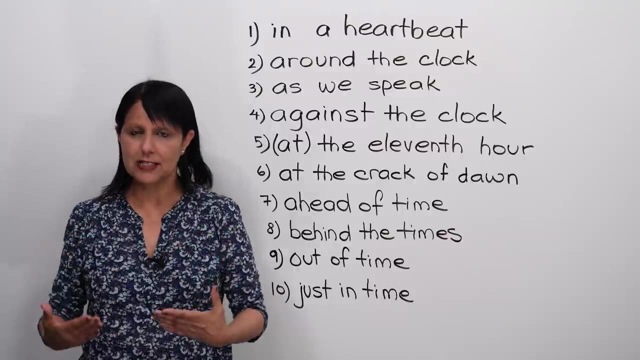 against the clock. Number four. okay, Now the way to remember these is to apply them, not just to listen, which is good. You could also note down. lots of our viewers are actually writing these down and making their own notes, making their own sentences, making their own examples. 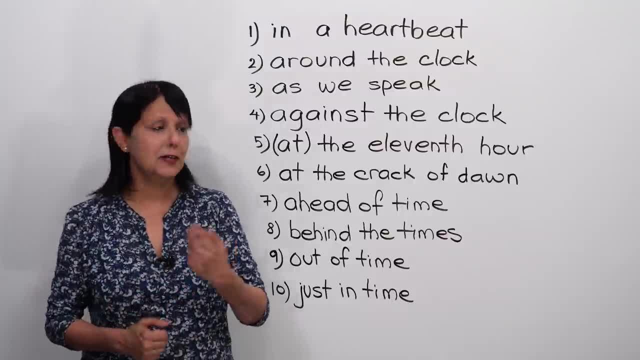 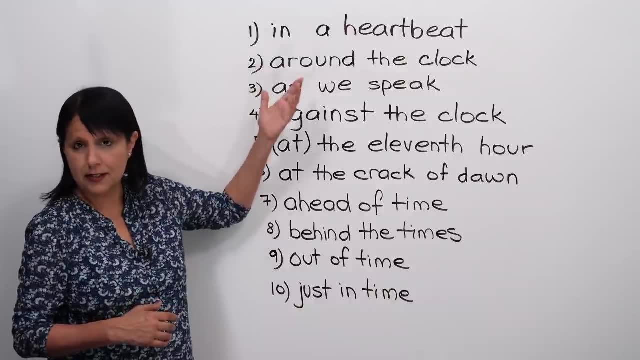 That's the best thing you can do. Apply it to your life. Think about a time when you were working against the clock. Think about a situation or a restaurant or something in your neighbourhood that's open around the clock- Things like that. Apply it. 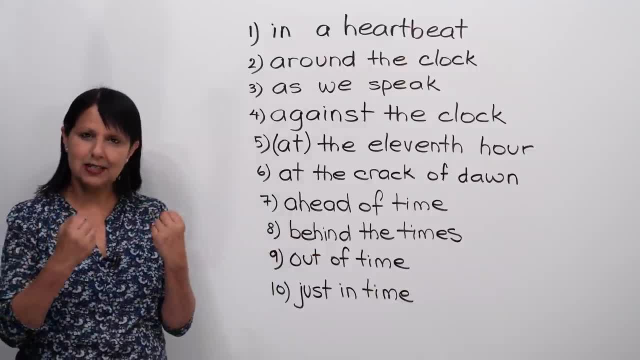 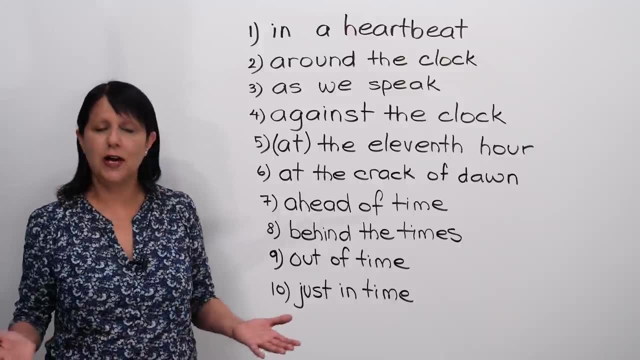 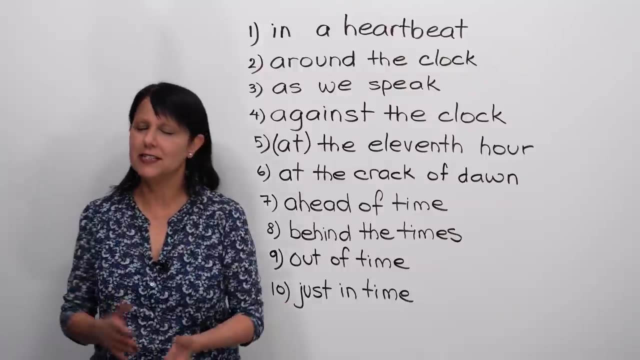 Apply it to your life, apply it to the life of people you know, to make it your own. so you really understand it. okay, Let's go on Number six. he woke up at the crack of dawn. okay, He woke up at the crack of dawn to study before his exam. 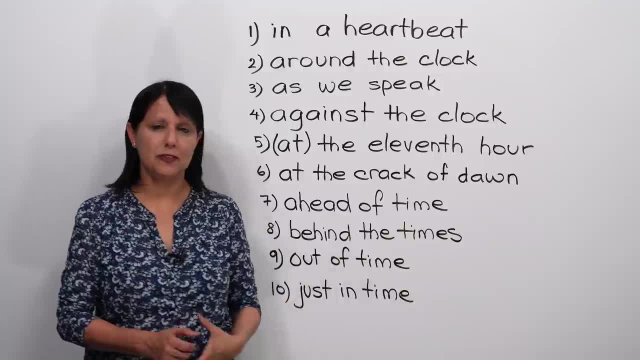 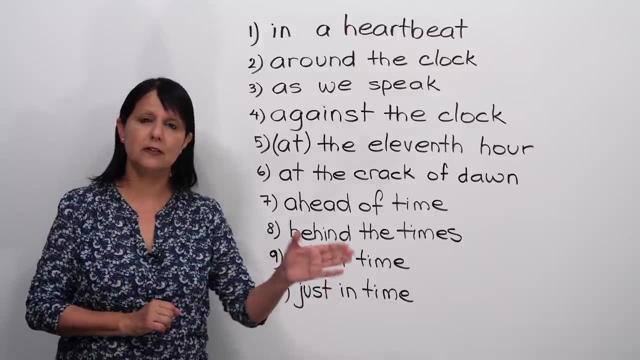 Any idea. So for that you need to know what the word dawn means. so dawn is when the sun is just starting to rise. Okay, It's very, very early morning, So he woke up at the crack of dawn means very early in the morning. 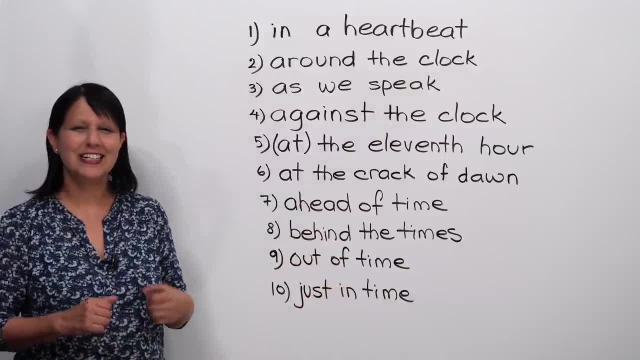 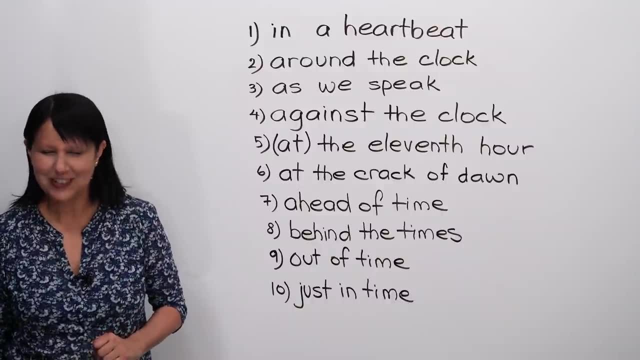 Like maybe I don't know four o'clock, five o'clock, whatever, it is okay, It just means very early in the morning. Let's look at the next one. Are you with me? Good, good, Number seven ahead of time. 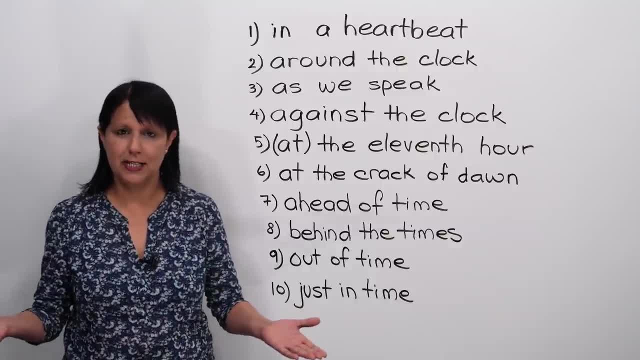 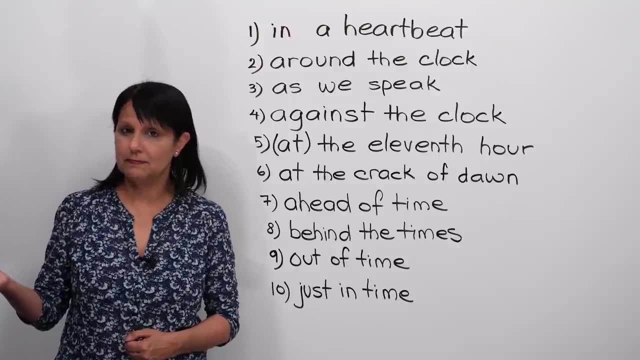 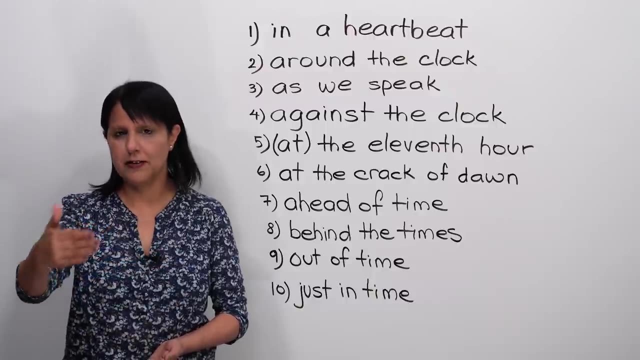 Okay. He always arrives ahead of time before an exam. She always arrives ahead of time before an interview. What do you think it means? Ahead of time means before the required time. She arrives early. In other words, it means early, okay. 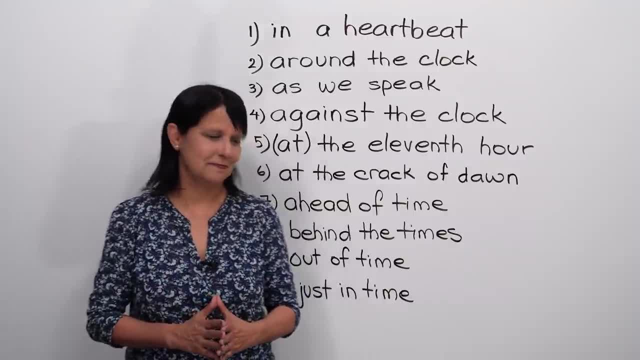 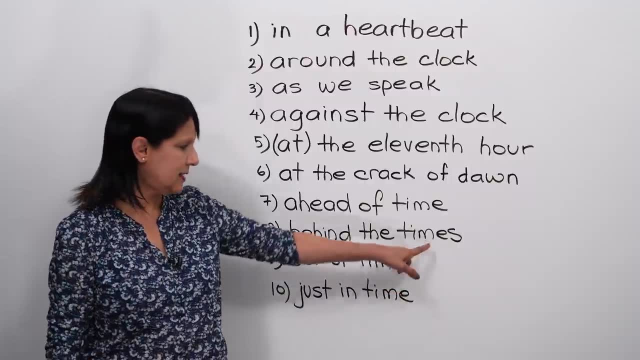 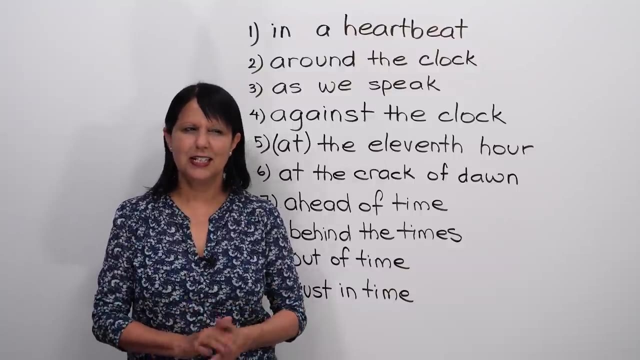 So ahead of time means early. Next, let's look at number eight behind the times. Okay, There's an S here behind the times, So we could say he's a little bit behind the times. he doesn't use email, he writes. 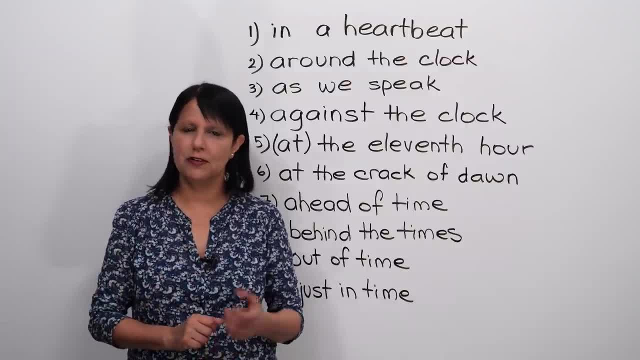 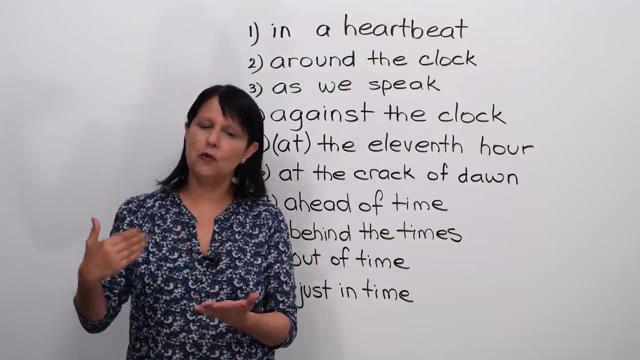 actual letters. he has a flip phone and not a smart phone. he's a little bit behind the times, Okay. That means not up to date, a little bit old fashioned, not using the latest technology, not having the latest ideas, Okay. 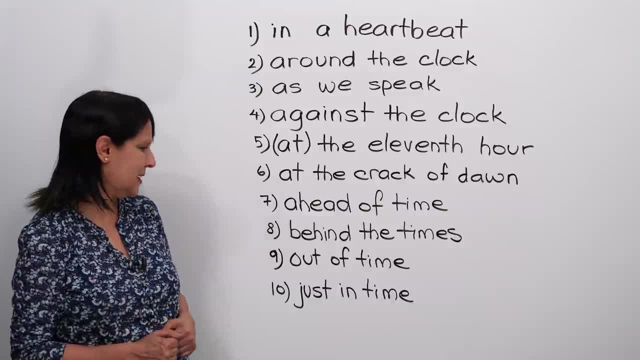 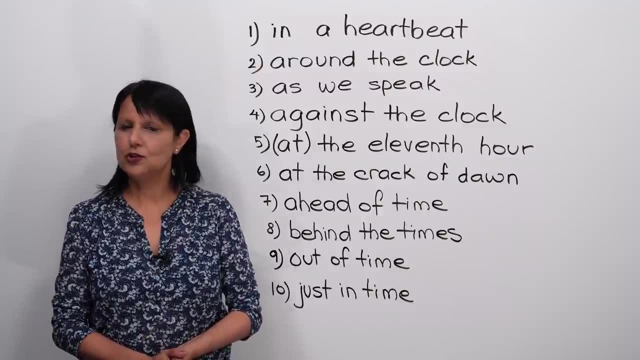 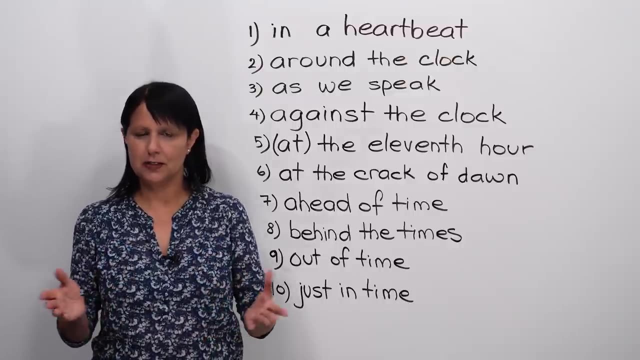 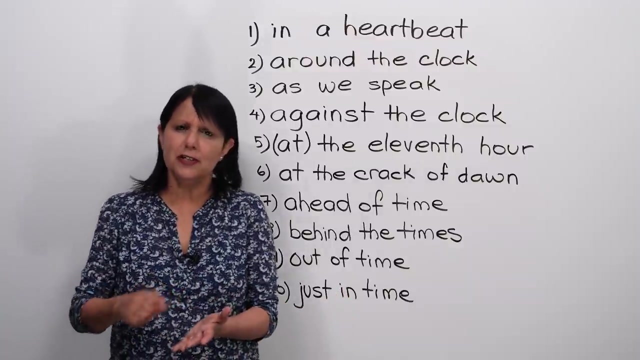 So this is behind the times. Next, Out of time. Let me give you an example. The teacher asked me to submit my exam paper right away because I was out of time. The teacher collected my exam paper and she said: I really wanted to finish, but she said: 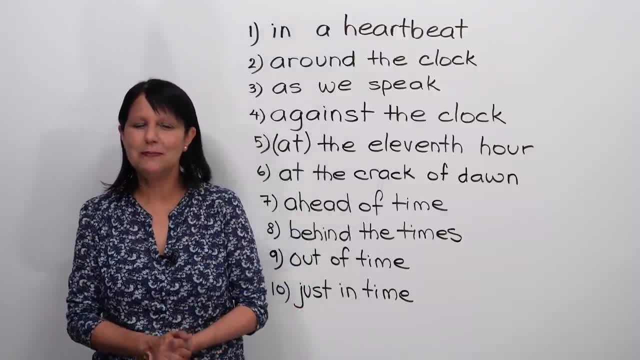 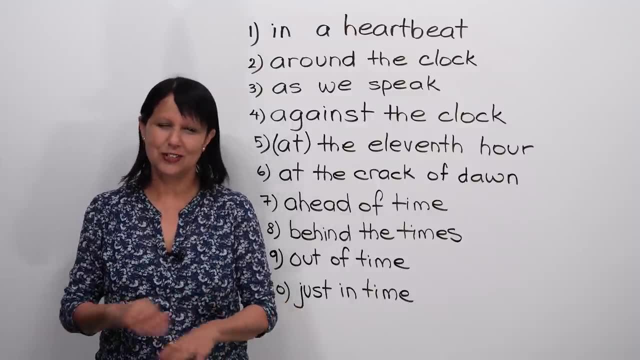 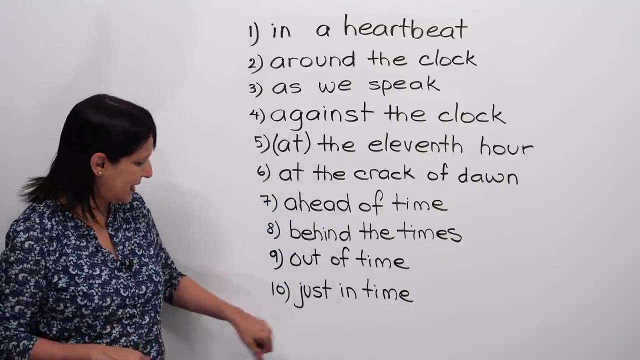 sorry, you're out of time. So what does it mean to be out of time, To not have any time left? Okay, No time left. You're out of time. You have no time left for something? Okay, Alright, and the last one, just in time. 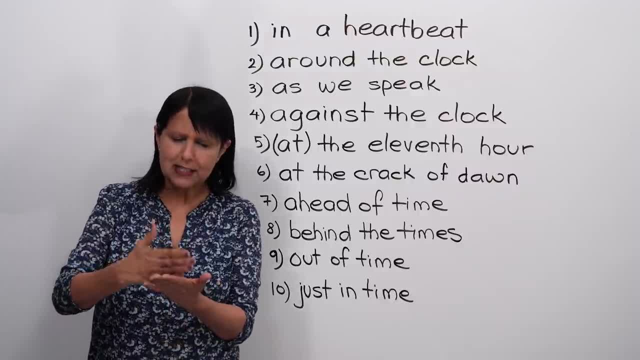 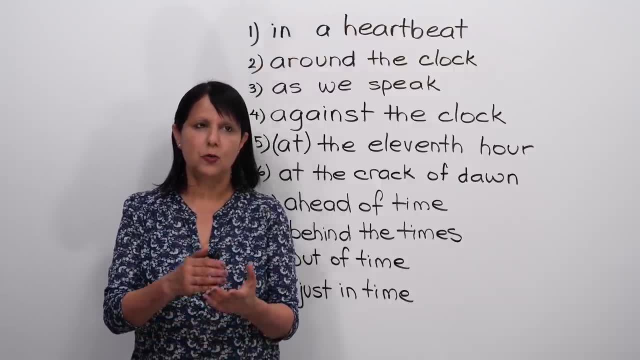 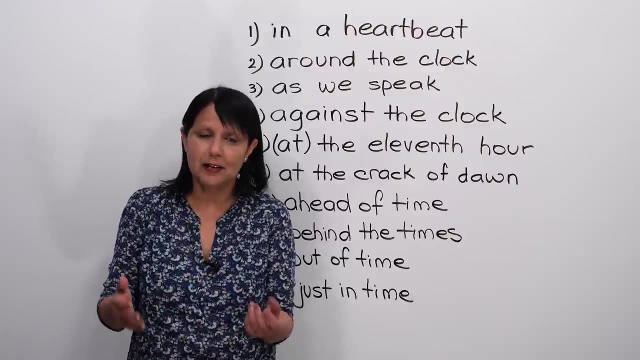 Okay, That means before, but at the last minute. For example, we arrived just in time to catch the flight, or we arrived just in time for the meeting, Or We arrived just in time for the wedding, otherwise we would have missed it. 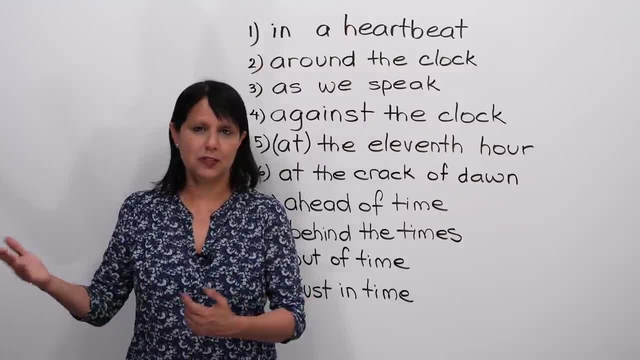 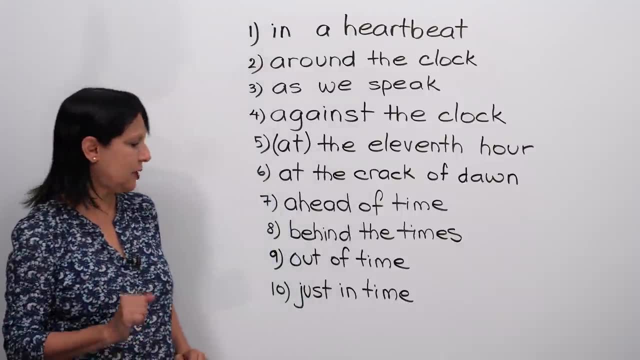 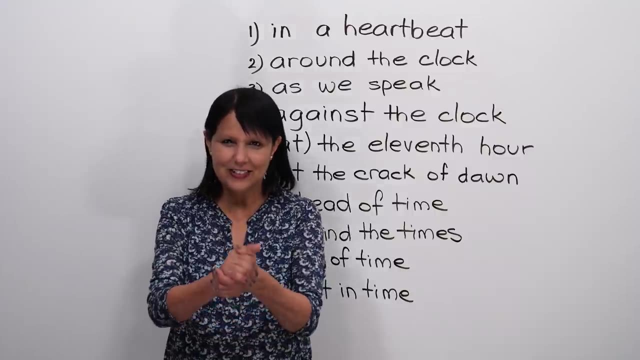 We would have arrived just in time for the movie. It was about to start. Okay, So just before something important was supposed to happen. if you arrived then, for example, then that would be just in time, All right, Good. 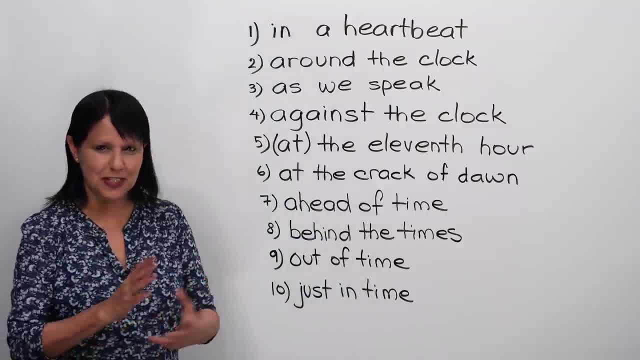 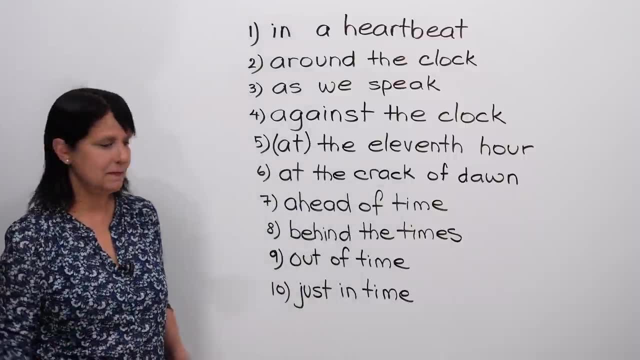 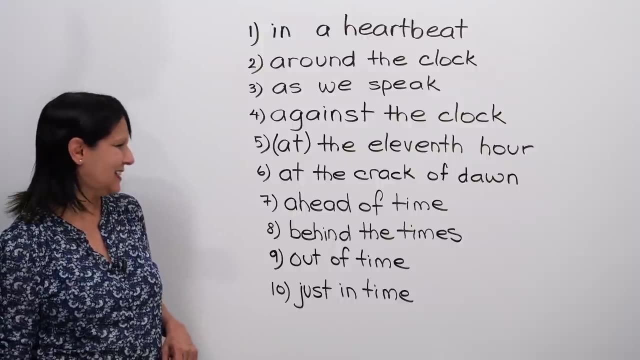 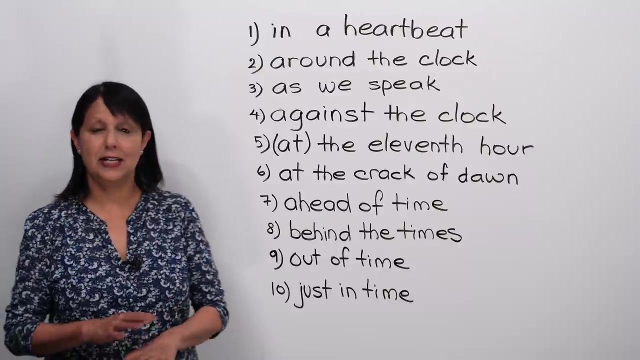 Are you still with me? Good for you. Let's review these a little bit. So, if someone always arrives early, they arrive when. Which of these last five? Have a look, They arrive ahead of time. Good, Okay, Very good. 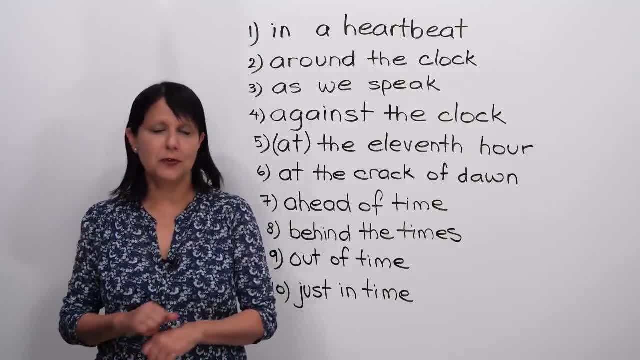 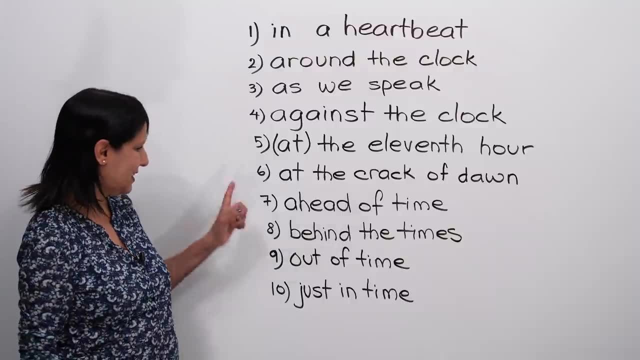 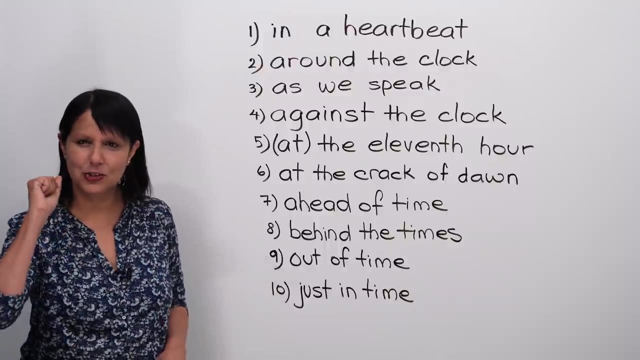 And you have no time left. you can't work on your exam paper anymore, you can't work on your presentation anymore. you have no time left. You are what? Which of these? You are out of time? Yes, I heard you. 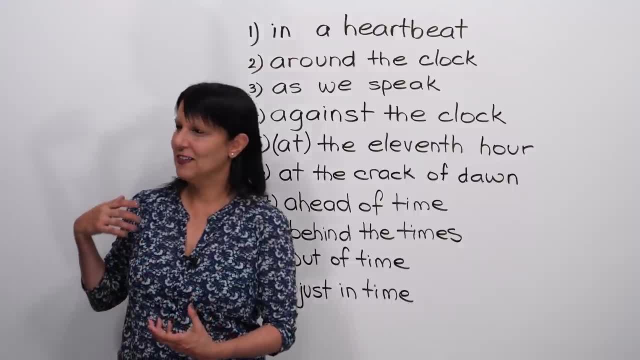 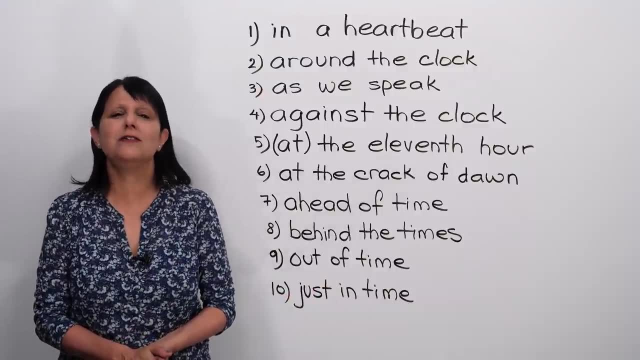 Good for you. All right, Let's suppose you have a lot of work to do so, Or you're just kind of a very super healthy person and you like to wake up really early in the morning, you like to meditate or you like to exercise or something like that. 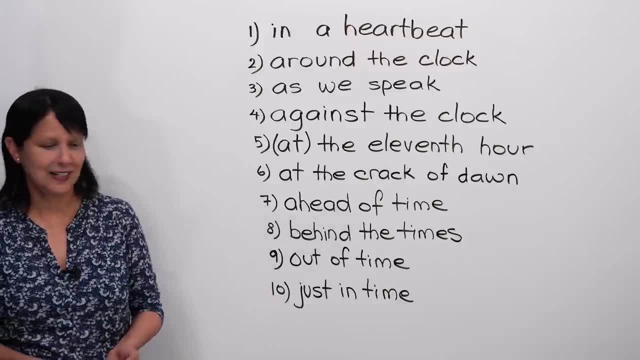 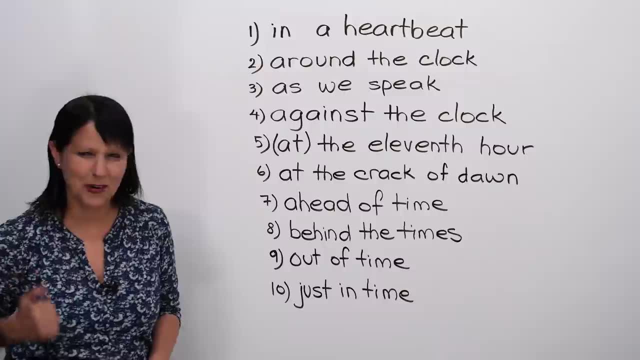 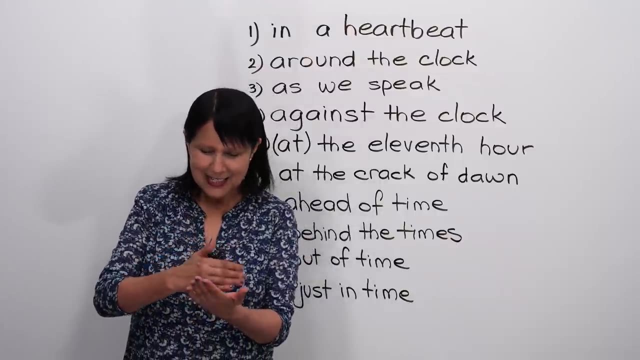 So when do you wake up? You wake up When At the crack of dawn, very, very early in the morning. Okay, And let's suppose you arrive somewhere before the last minute, before something important happens, then you arrive. 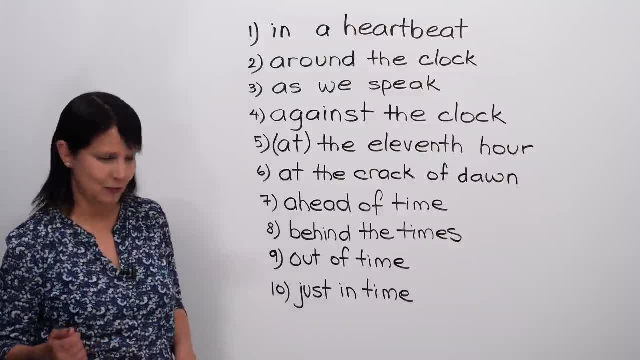 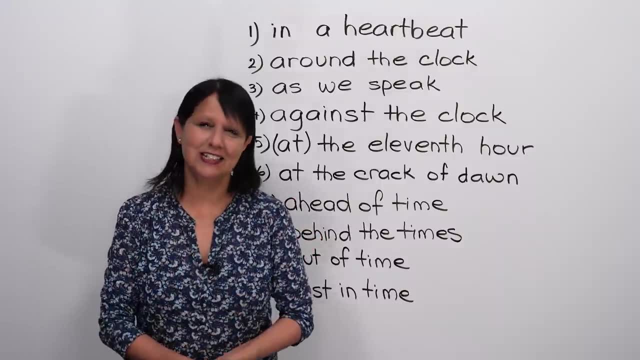 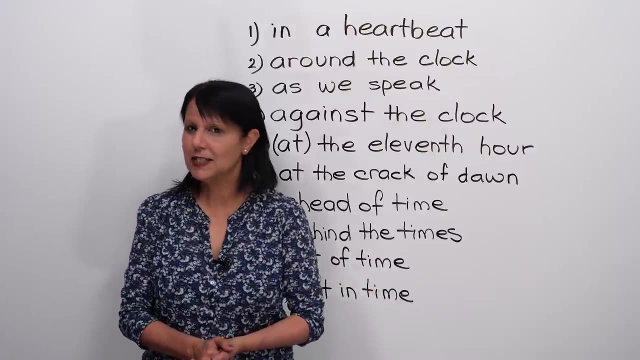 Which one? Just in time, Right? And what do we leave out? Okay, All right. So Let's suppose somebody is not using the latest technology, not using the latest equipment, and so on. that person would be what Behind the times.